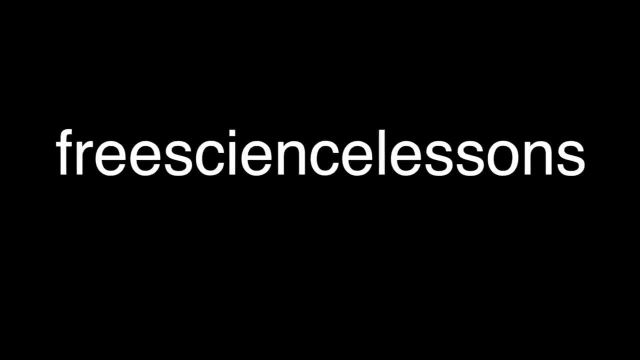 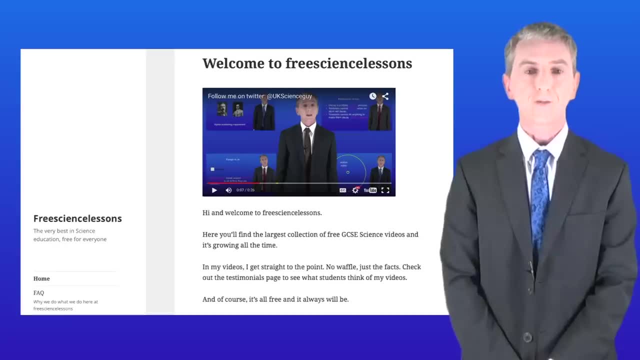 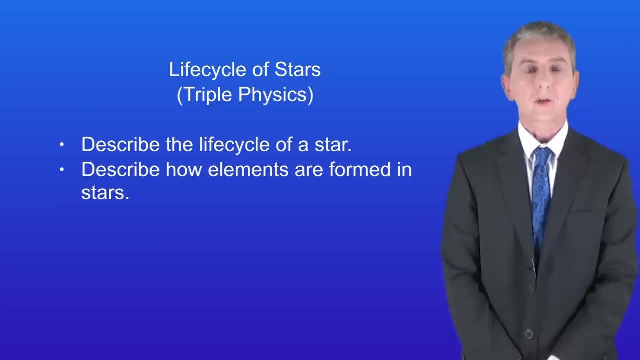 Hi and welcome back to freescicelessonscouk. By the end of this video, you should be able to describe the life cycle of a star. You should then be able to describe how elements are formed in stars, and this is for triple physics students only Now. I should point out that there's quite a 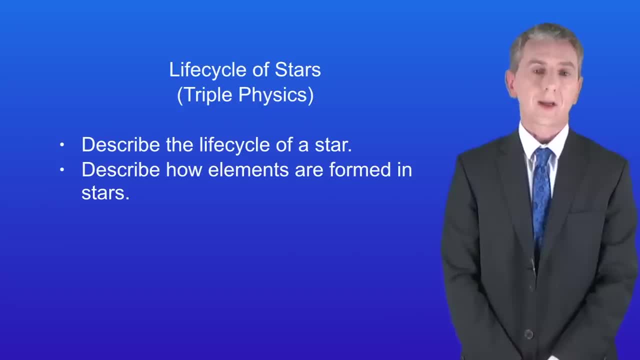 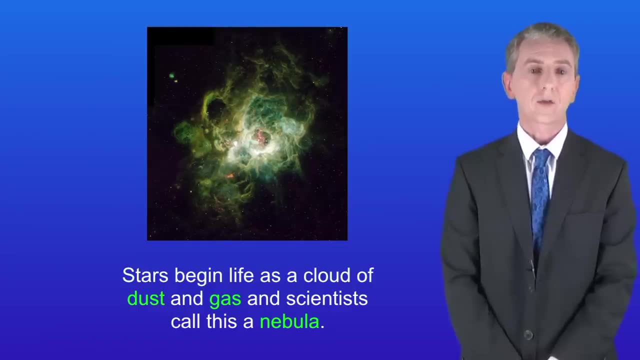 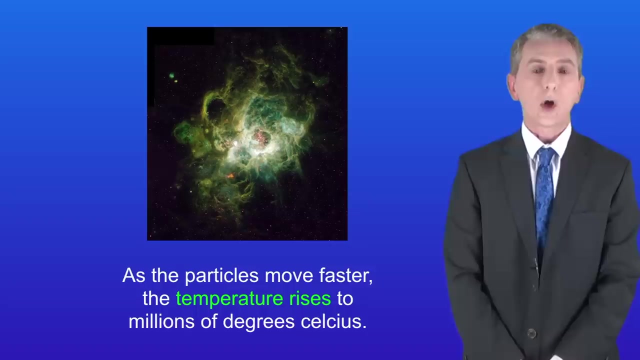 lot to learn here, but it's worth making the effort. It does come from the exams and you are meant to know the specific details. As we said in the last video, stars begin life as a cloud of dust and gas, and scientists call this a nebula. Gravity causes the cloud of dust and gas to collapse As the 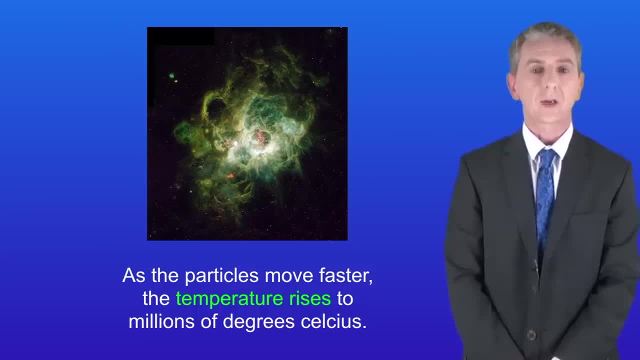 particles move faster. the temperature rises to millions of degrees celsius. This early stage is called a protostar. If the temperature gets high enough, then hydrogen nuclei join together to form helium nuclei. This process is called nuclear fusion, and we looked at nuclear fusion in an 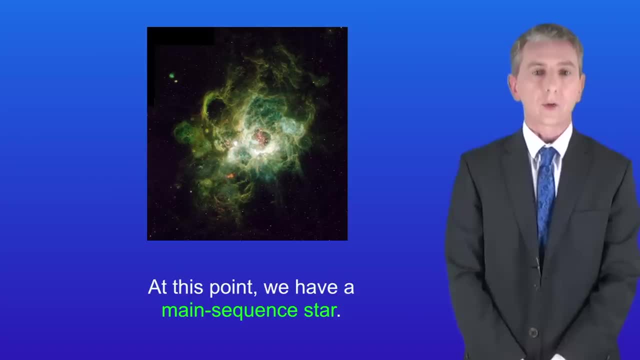 earlier video. At this point we've got a main sequence star. Nuclear fusion releases a huge amount of energy and stars can stay in the main sequence for a very long time. But what happens next depends on the size of the star and you need to learn these stages. We're going to start by looking at what 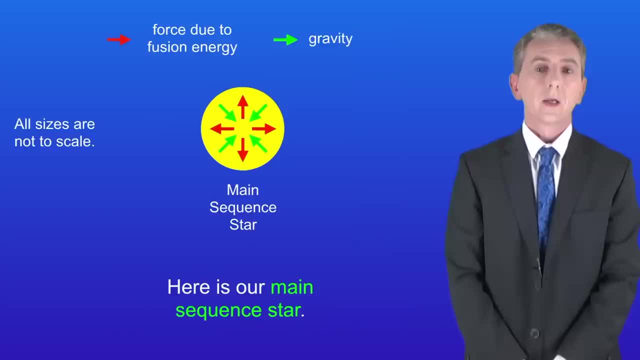 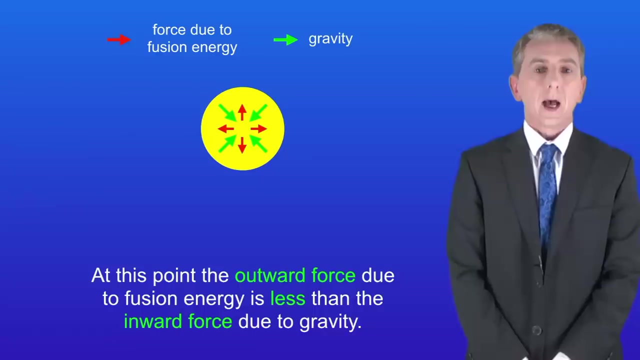 happens to stars that are about the same size- our Sun. So here's our main sequence star. As we said before, in a main sequence star, hydrogen nuclei fuse together to make larger nuclei such as helium. Now, at some stage, the hydrogen in the star begins to run out. At this point, the outward force 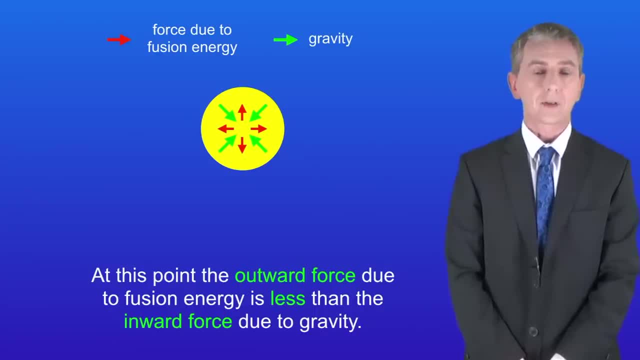 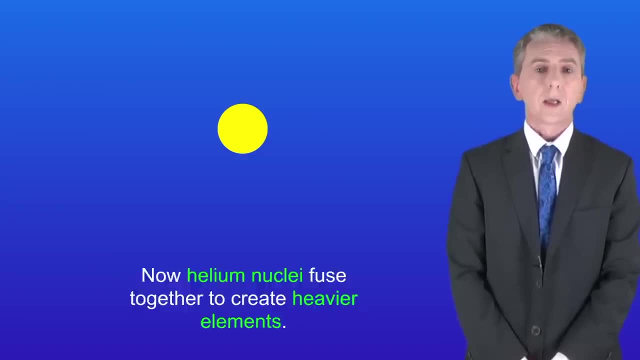 due to fusion, energy is less than the inward force due to gravity. This causes the star to collapse inwards. The collapse of the star causes its temperature to increase. Now helium nuclei fuse together to create heavier elements and the star expands to form a red giant. At some point, the red 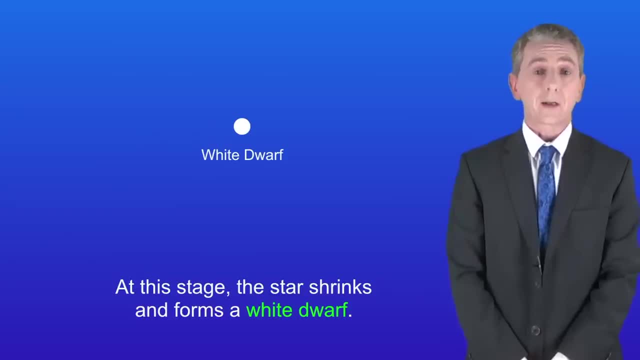 giant stops fusing helium. At this stage the star shrinks to the right of the star. This causes the star shrinks and forms a white dwarf. Because the white dwarf's no longer carrying out fusion, it gradually cools down. Eventually it stops releasing any energy and it forms a black dwarf.